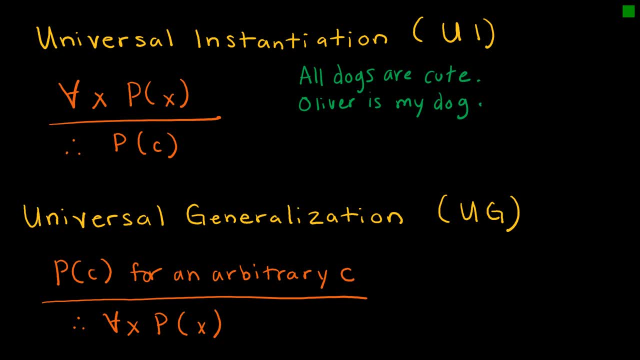 My dog, Oliver, is an element in the domain and therefore I can say that P O we'll just use O for Oliver, which essentially means Oliver is cute. The universal generalization is essentially this: rule backwards. So if I tell you that P of C is true for an arbitrary C, 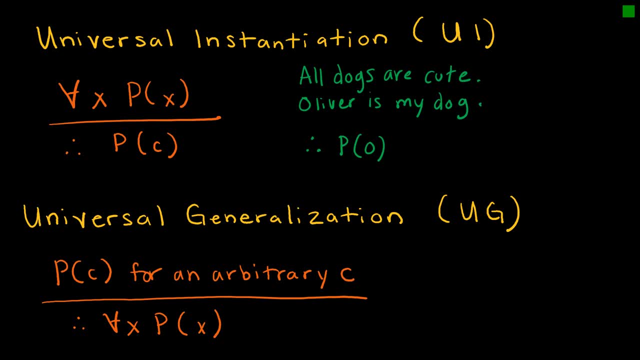 then essentially I'm saying that P of C is true for an arbitrary C, So I'm saying it is true for all values. Now, the important thing to remember with this rule is that we're talking about an arbitrary C, or essentially we're saying, if we pick any old value from the domain, 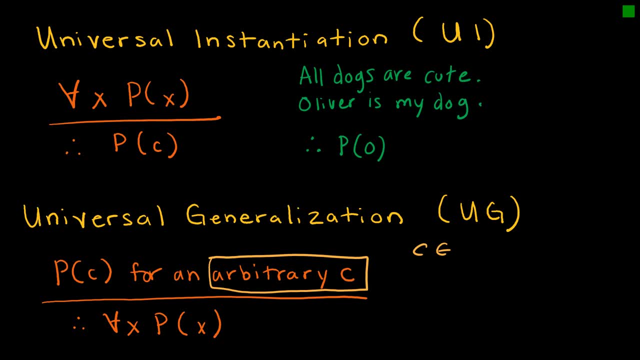 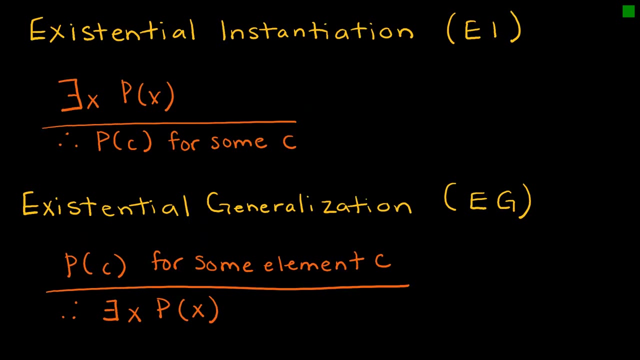 so some C value that belongs to our universe, then if it's true, no matter which value we choose, essentially we're saying it's true for all values in the domain. Our next two rules should flow very easily from our last example, and that is existential instantiation and existential generalization. 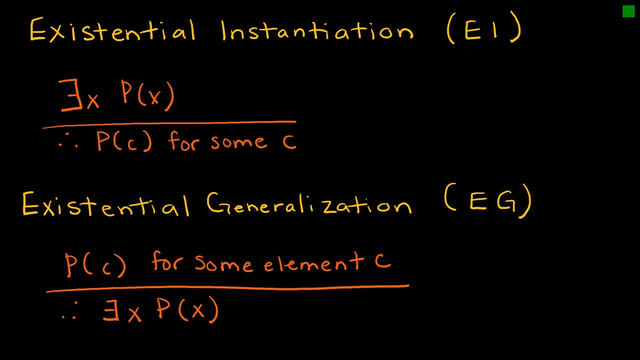 So again, my first one is saying there exists some X such that P of X. so we're saying there is some X such that P of X. there is some value that makes this true. therefore, I can say that it's true for some specific value. 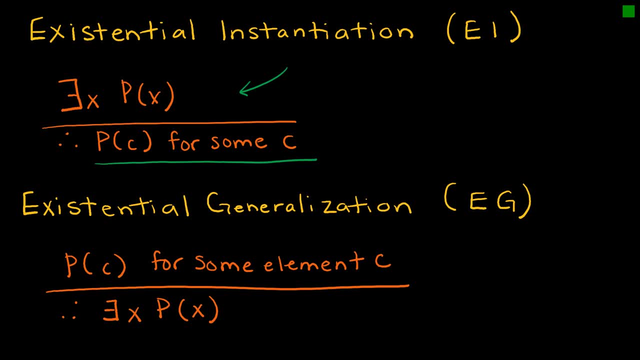 And that's really just the definition of existential, Same thing for existential generalization. it's just this backwards. So we're saying if P of C is true for some element of C, then we can say there exists some element X such that P of X is true. 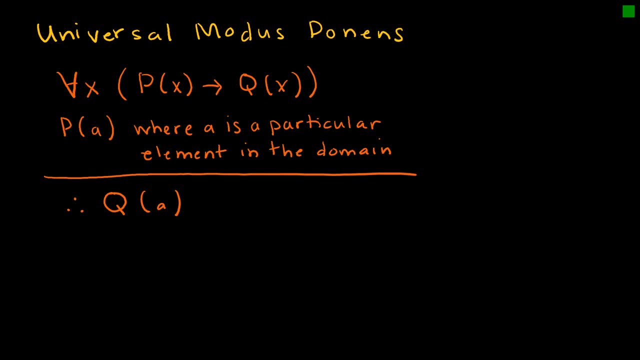 And, of course, our very, very favorite one that we use so very often: modus ponens. this is universal modus ponens. So, for all X, if we know that P of X implies Q of X and we know that P of A is true, 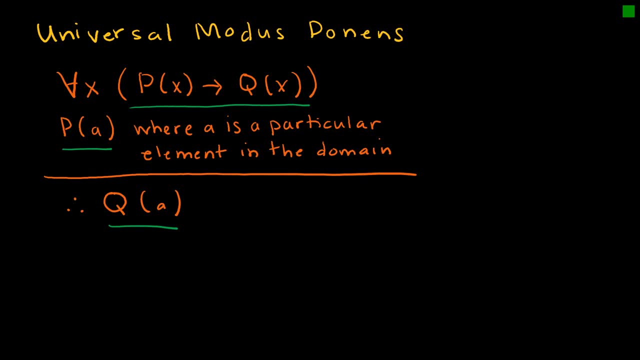 therefore we know Q of A is true. So again we've got that if-then statement and whenever we have that if-then statement and we can show that the first part is true, then we can show that the second part is true. 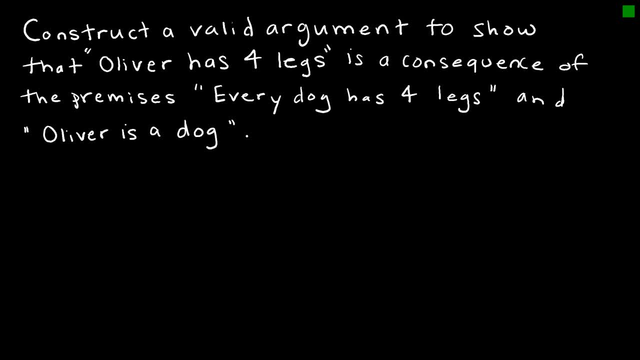 Let's see if we can't work together to construct a valid argument to show. if we know the premises- every dog has four legs and Oliver is a dog- we can conclude that Oliver has four legs. So the first thing we want to do is come up with some predicate statements. 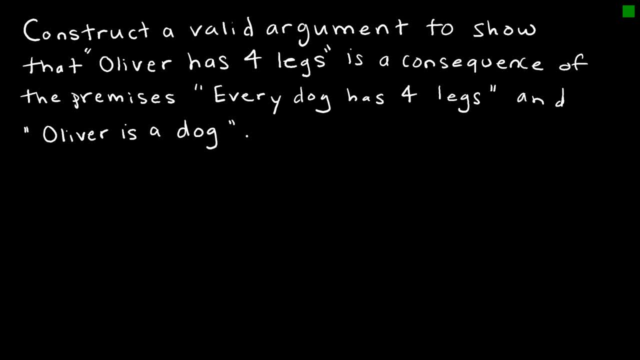 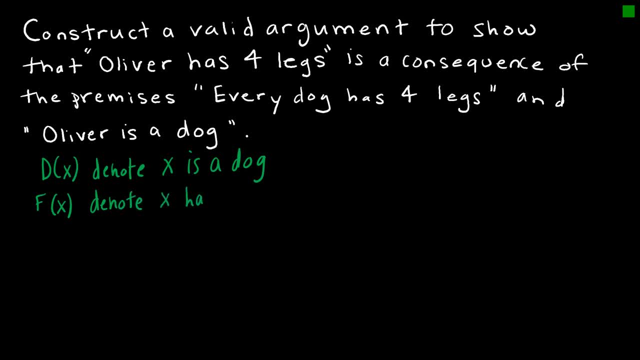 X has four legs. So now that I have my predicates, I want to be able to write my premises using those predicates. So every dog has four legs can be written, and again, this is saying every dog. so that's for all X. that belongs to the domain. 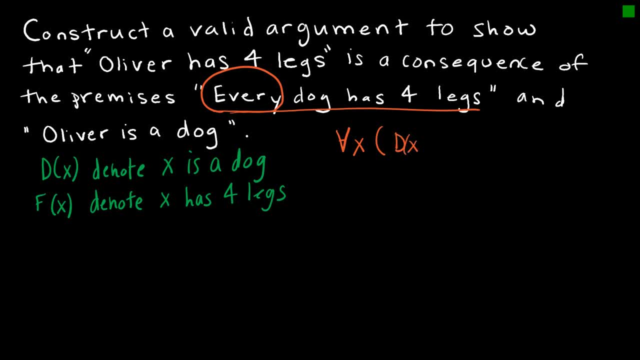 We're saying if it is a dog Then it has four legs. My other premise says Oliver is a dog And so I'm going to say D-O, O for Oliver, So X is a dog. I'm saying D-O, which means O is a dog or Oliver is a dog. 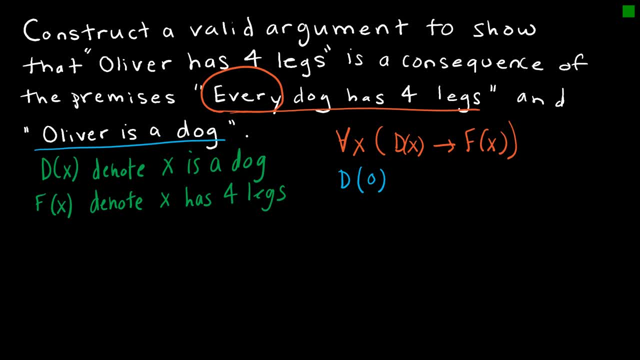 So these are my two premises, and now I'm going to construct my argument. So let's see how we do. Number one I'm going to use for all X. if D of X, then F of X, And that is a premise that was given to me. 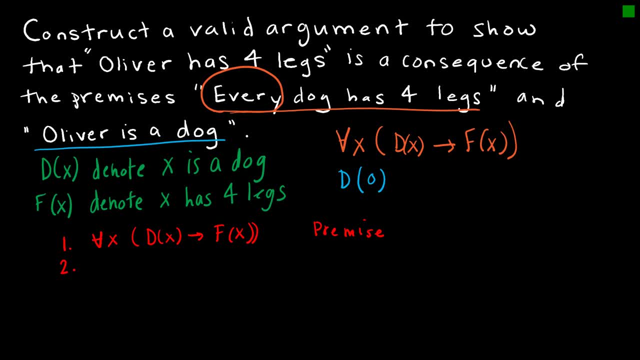 Now, what we just learned is that if that's a premise, if that is true, then I can say: I mean, if it is true for all of X, then I can say it is true for a specific X. So if Oliver is a dog, then Oliver has four legs. 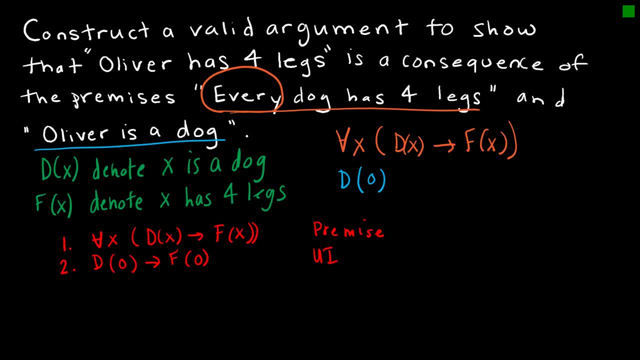 And what's the reasoning? Universal instantiation from one. Now I can use D-O, Which of course was another premise, that Oliver is a dog. So now I've used both of my premises And because of that I can conclude F-O. 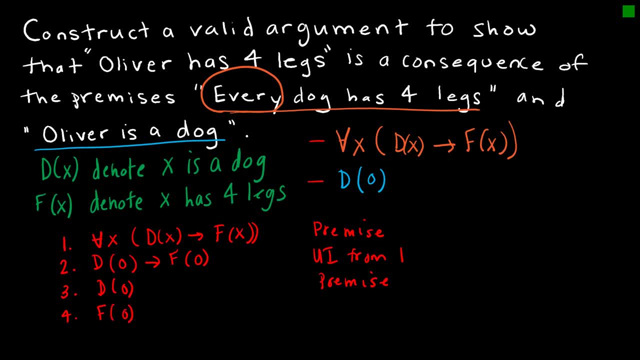 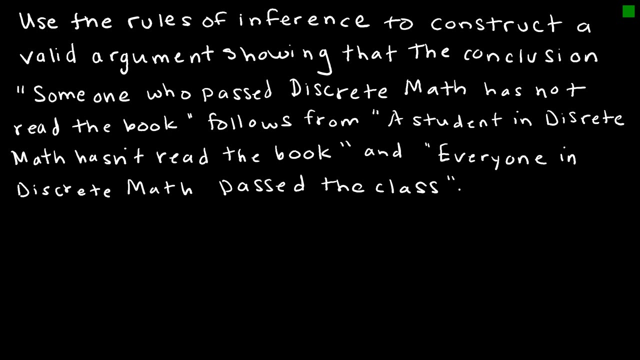 which, of course, is that Oliver has four legs, And that's modus ponens using two and three. Here's another question for us to try, and this one is a little bit more complicated. If you want a challenge, go ahead and press pause right here and try this question first. 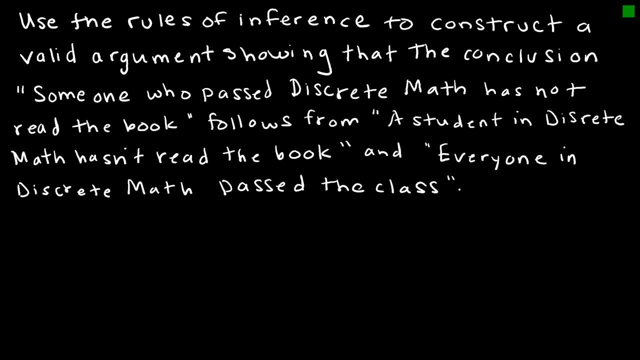 If you just want me to go through it with you, then that is what we're going to do right now. So we are going to use the rules of inference to construct a valid argument showing that the conclusion- someone who passed discrete math has not read the book. 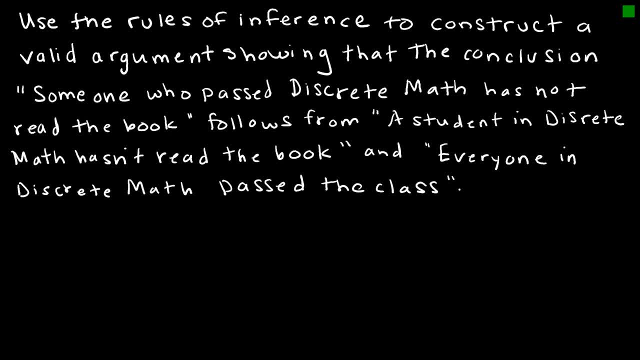 follows from: a student in discrete math hasn't read the book, and everyone in discrete math passed the class. So the first thing I want to do, as always, is to come up with which predicates I will use, And in this case I'm going to let D of X denote. X is a student in discrete math. 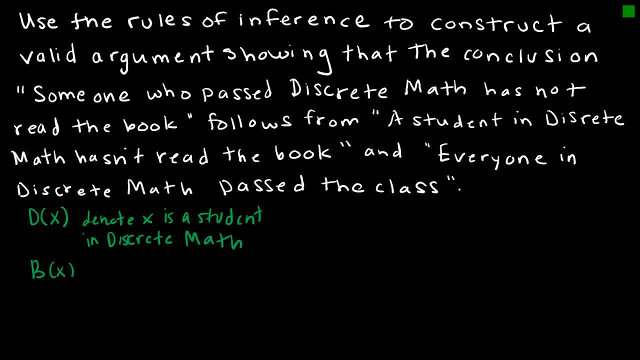 Then I'm going to let B of X denote that X read the book And lastly, I'm going to let P of X denote that X passed the class. So those are all of the things that I know is something about reading the book. 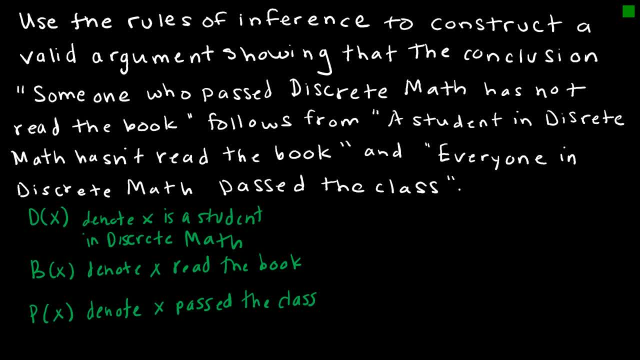 passing the class and obviously that that person is in discrete math. So let's see if we can't take some of these statements and write them using predicate logic, So we'll get to this one here at the end. Let's start with a student in discrete math hasn't read the book. 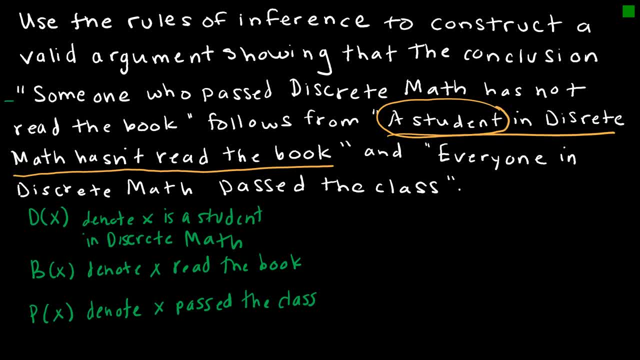 So we're saying a student, which means there exists a student, such that now we're saying it's a student in discrete math and they have not read the book. So a student in discrete math would be D of X and they're in the class and haven't read the book. 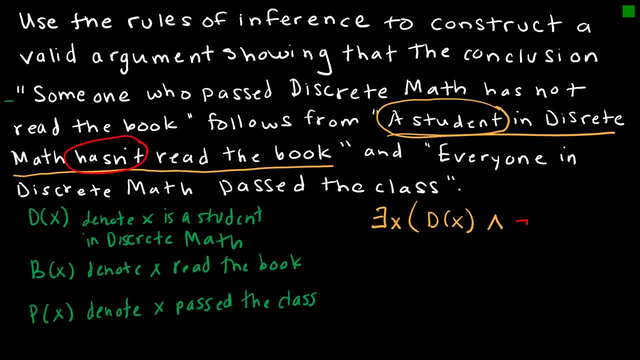 So remember, if it's a negation here, then I have to use that negation here, So not BX. So that's that first statement. Now let's take a look at everyone. in discrete math passed the class. So everyone tells us that for all students who are in the class. 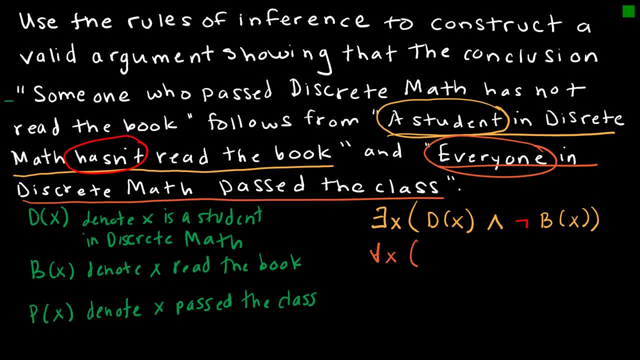 so that's a for all X. what do we know? The student is in the class and passed the class. So if the student oops, not C of X, sorry, not class, but discrete. So if that student is in discrete math, then that student passed the class. 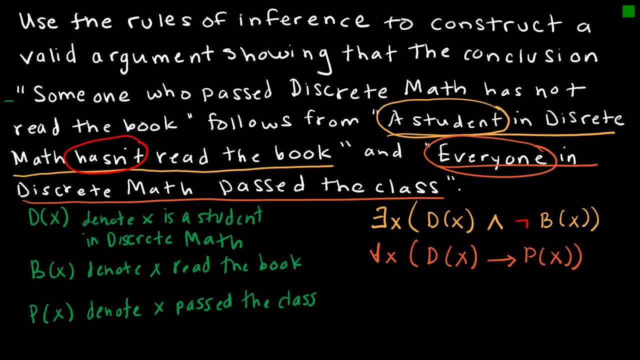 So, for all of X, D of X implies P of X, And what I'm trying to get to is right here. Someone who passed discrete math has not read the book. So what is my conclusion going to be? I want to prove that there exists some student X such that they passed the class. 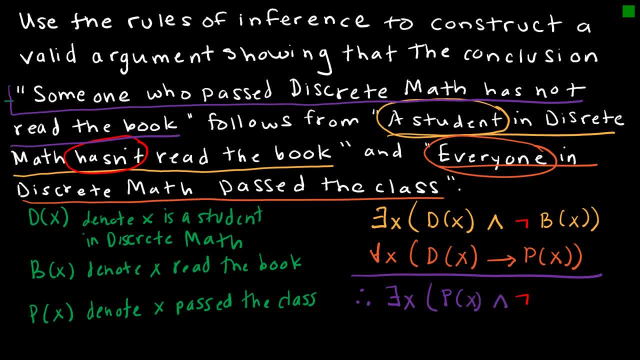 and they did not. Now I haven't proved anything yet, but what I've done so far is I have organized my thinking so that I know what my premises are and what I want my conclusion to be. So now I'm going to move on to actually doing this proof. 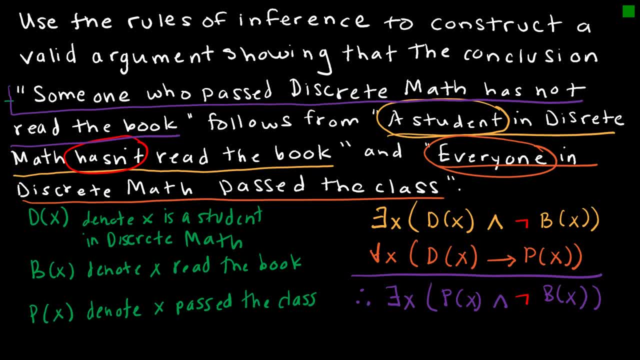 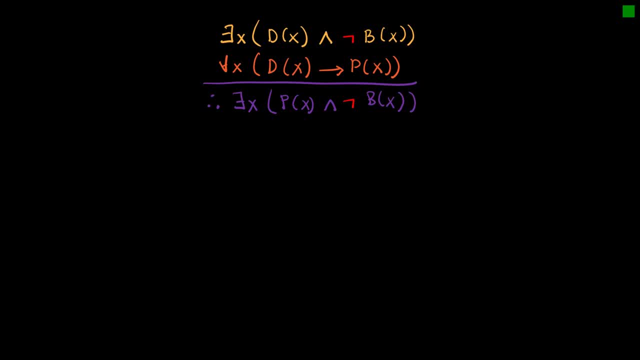 Okay. so now that we know what we know and where we're headed and what we're going to do, we're going to move on to the next step, which is going to be proof. Okay, And what we know is, of course, our premises, and where we're headed is here in our conclusion. 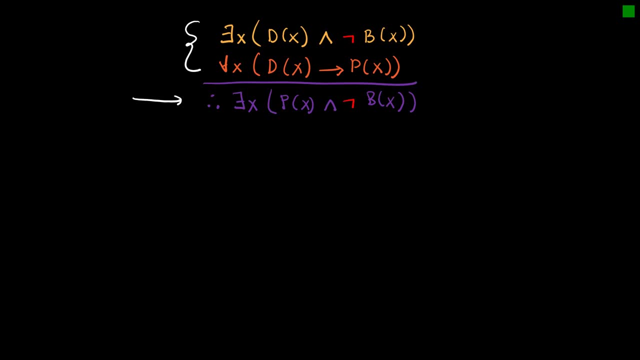 Now I want to figure out a valid argument using my rules of inference that helps me to use those two premises to arrive at the conclusion. Now, before I start all willy-nilly into my proof, I know that this is where I want to end up. 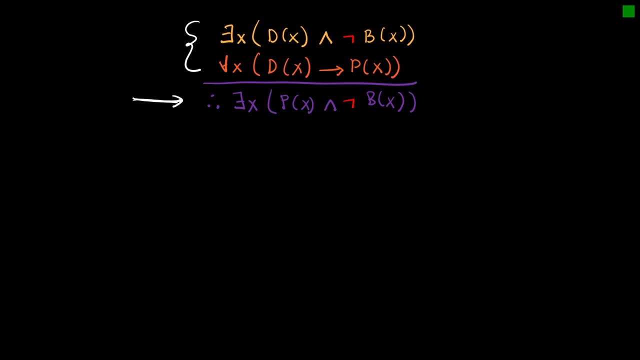 I want to end up at the conclusion. Well, how could I possibly end up at a conclusion that says there exist these things unless I can prove it? Well, how could I possibly show that pt is correct? Maybe I can show that p of x is true for some x, some x, because there exist in x. 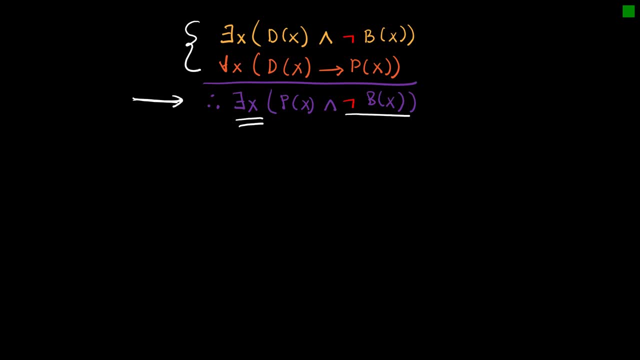 and that not b of x, is true for that x. So let's see how we get there. We're going to start just by using our first premise that there exist in x such that d of x and not b of x. 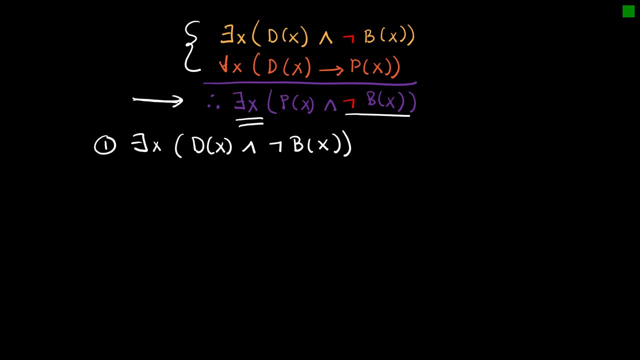 they're in the discrete math class and not b of x means that they're you know? not, they have not read the book, but i think that actually makes it a little bit more confusing, and the reason for me being able to say that is a premise. so that's where we are so far. again, keep in mind where we're. 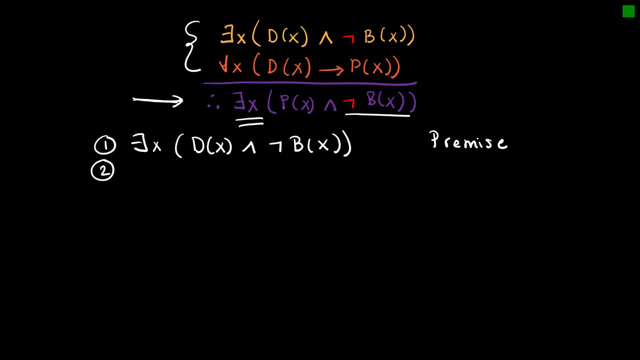 heading, and so what i don't like about that first premise is that there's a quantifier, and quantifiers are difficult to deal with. so that's why we have those new rules, and one of those new rules says that if it's true for some element in the domain, then i can say it's true for a specific. 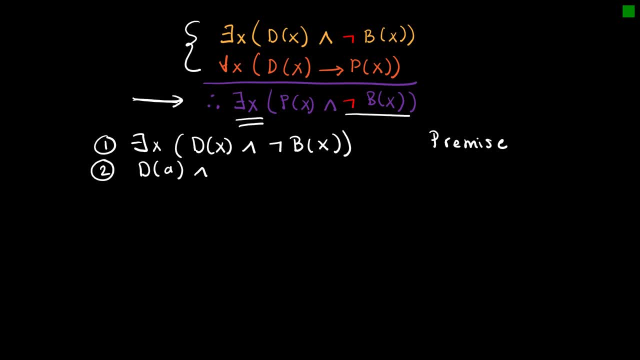 element in the domain, there exists some element a, such that d of a and not b of a, and that's ei existential um instantiation from one. so basically, i just said, hey, it's true for this one element. now, remember that this is an and, and when we have an and, 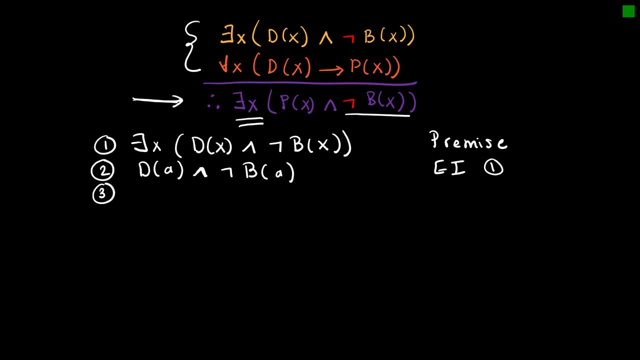 we can say: therefore, it's true for each one of them. so i'm going to start by just saying d- a is true, by simplification. now you might say: well, why? why did you choose that? well, because i know that i'm going to end up talking something about d of x or d of a, and so this just tells. 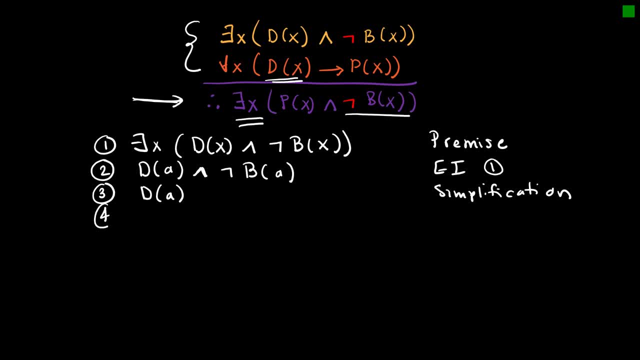 me that it's true and that's going to help me further down the line. so now, what am i going to do? i'm just going to give that second premise, whoops for all: x. d of x implies p of x, and that is a premise. and i bet you can guess what we're going to do now because again, i've got this quantifier i. 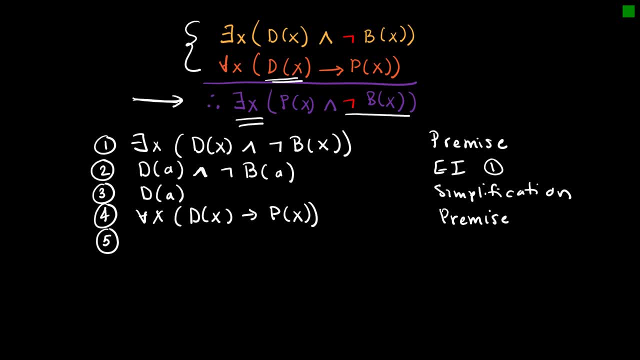 don't love the quantifiers. so i'm going to say now that d of a implies p of a. so i'm just saying specifically for one element in the domain, and that's universal instantiation for four. well, now what? now i know that if d a is true, then p a is true. and guess what? probably cares letting me pick one. all right, i don't know if this is true, i know d is true, so i'm going to take 4 and 4 together, l 4, and I have two canos into one of the islands level. you might want to. if data is true, i use thejego of I n. what number of theparameters of current conditions are n equals C to Caleb, 4 or P? go by and number of Flo dropping into d is c of a. now that will be four. which is d or a in the domain? and that's universal instantiation for 4. for well, now what? now I know that if d a is true, then pa is true. and guess, 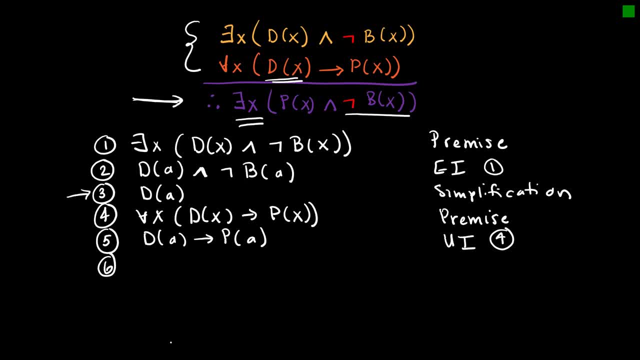 what I already showed up here, that dA was true. so that's going to be that pA is true and that's good old modus ponens with 3 and 5.. So 3 and 5 with modus ponens tells me pA is true and that. 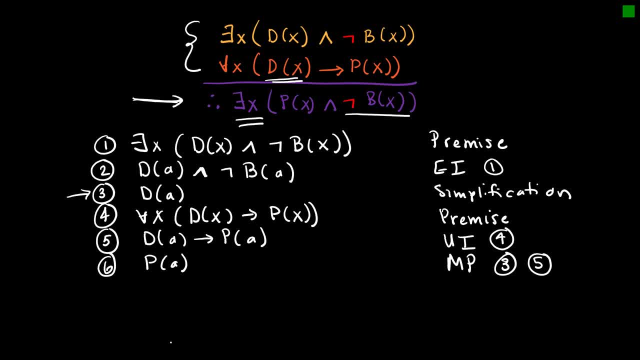 makes me happy, because look where I'm trying to head up here. I'm trying to get to p of x or in this case, p of A and not b of A, so that I can get to that final conclusion statement. So of course, for 7 I'm going to say: not b of A, but I can't just decide: not b of A, but I can. 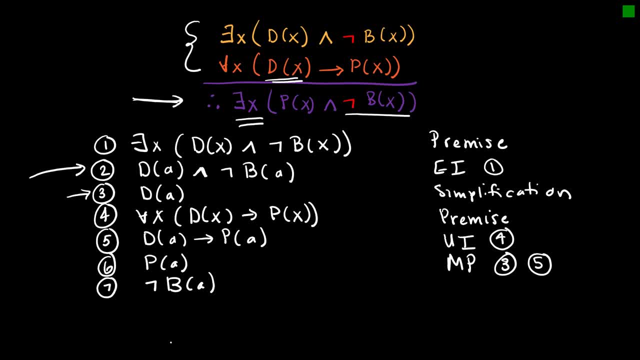 use it from 2.. Remember 2,? we said both of those things were true for that element A and therefore this is just simplification from 2,, just like we did before. So I'm going to use it from 2, and I'm going to use it from 2, and I'm going to use it.